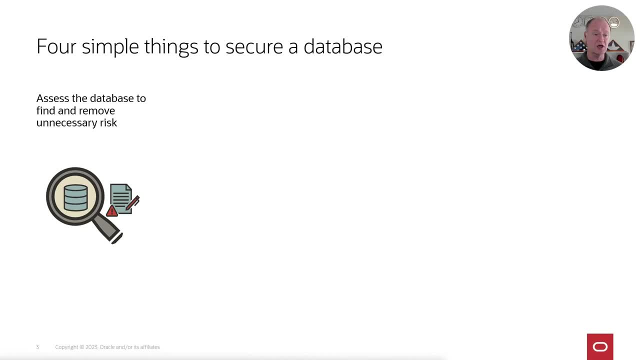 standpoint and they can introduce unnecessary risk. You want to find those settings And if you are accepting additional risk, you want to make sure you do that with your eyes open. You don't want to be blindly accepting things and not knowing what's going on. So you assess your database to 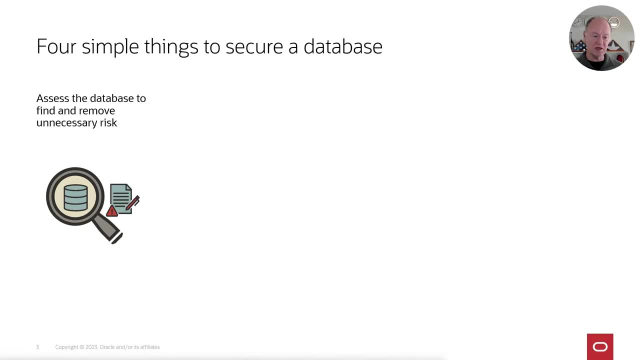 remove unnecessary risk. The second thing you do is obvious in today's world: You need to encrypt your data. Encryption is a fundamental security control, And that means your data as it travels over the network. It also means your data as it is stored within the database. All data should be encrypted. 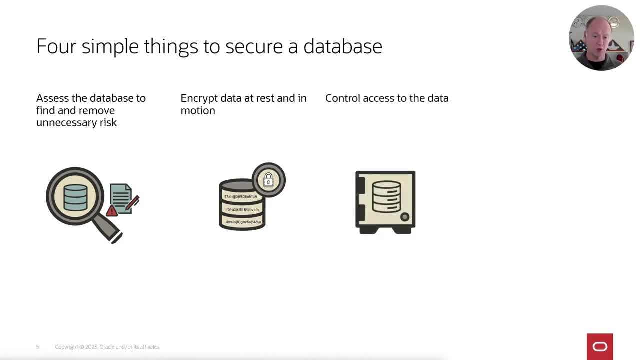 pretty much all of the time You need to control access to the data You don't want. well, in most cases, everyone who can access your system shouldn't be able to access all of the data within that system. They should be able to see the data that is relevant to whatever business. 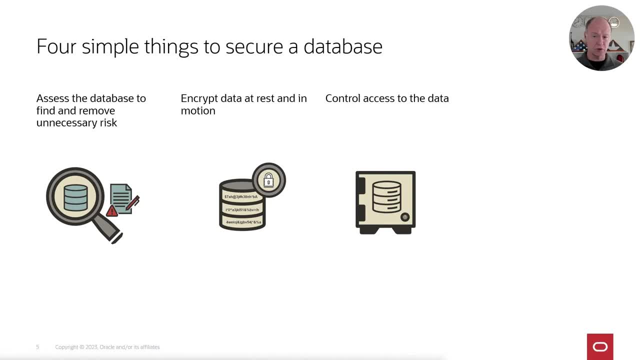 thing they're doing And they should be able to see the data that is relevant to whatever they have to do, not all of the data. So you control access to the data And then the final thing you've got to do is you've got to plan for failure. The bad guys are out there. They are. 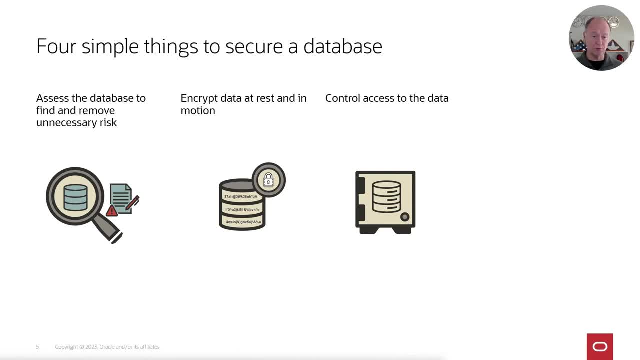 definitely trying to get at your data. You want to assume that they are going to be probing your defenses And you want to audit what's going on in your database, for two big reasons. One of them is: maybe through your auditing you catch what's going on before something bad happens and you're 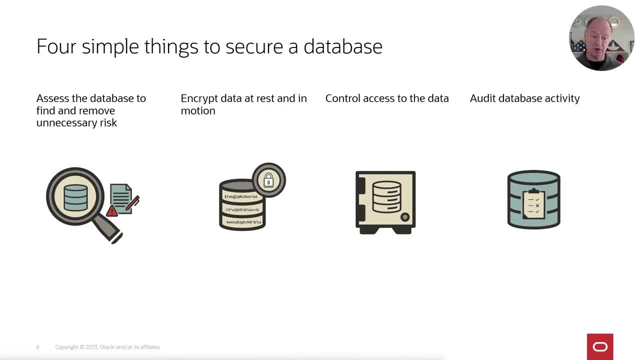 able to stop it from happening. Or maybe you don't catch what's going on, but later you can go back and reconstruct what the bad guys did so that you can determine what the amount of damage was. What was the blast radius of this type? 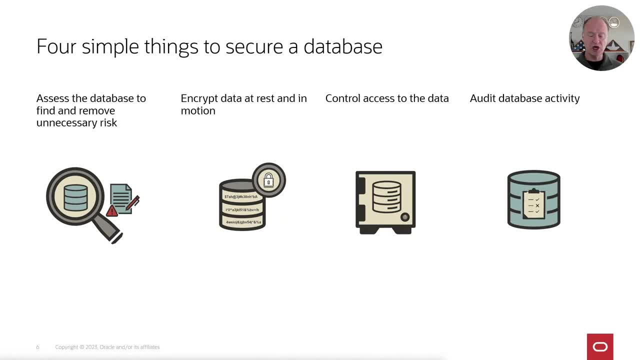 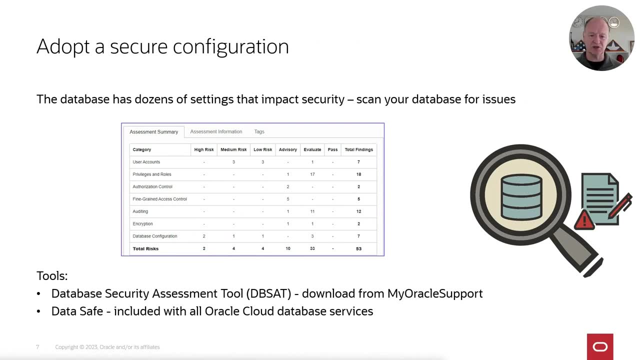 of attack. Let's take these four different things individually. We'll start with adopting a secure configuration. Like I said, the database has dozens of settings that impact security And you want to make sure that you're controlling your configuration so you don't expose additional risk. Now there are 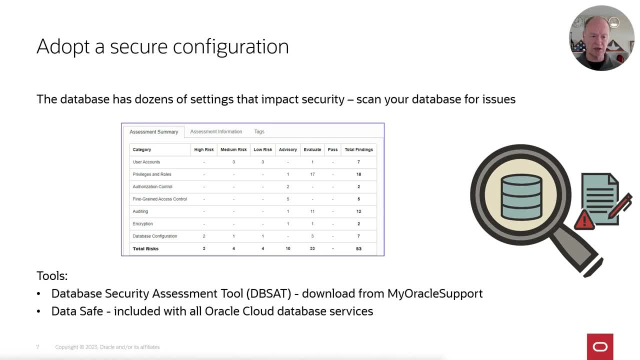 a couple of tools in your toolbox that can help with this. All right, One of them is the database security assessment tool. Others include things like data save for enterprise manager configuration dashboards, But we're going to start with the database security assessment tool. It's basic. 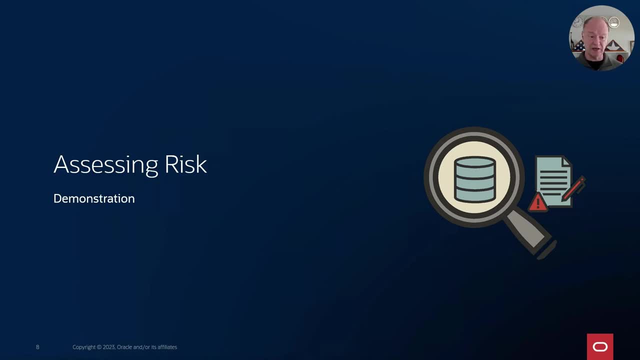 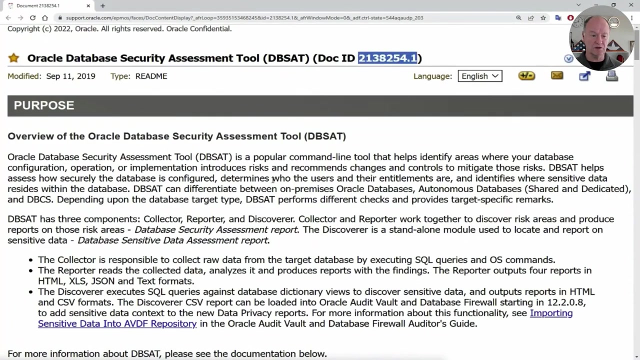 fundamental, very, very easy to get to. It's a command line utility. that really is a lowest common denominator. If you have access to your database, you can run the database security assessment tool. All right, So let's look at this. We start by going to my Oracle support. We go to the support. note that 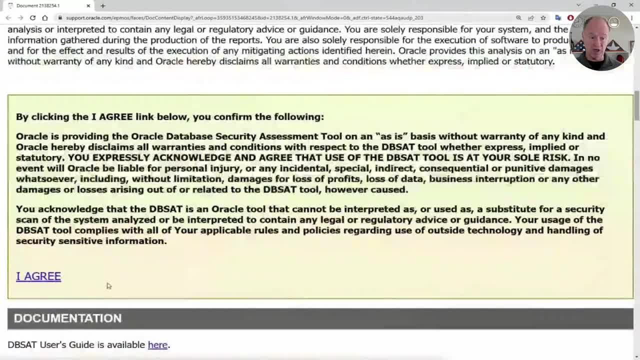 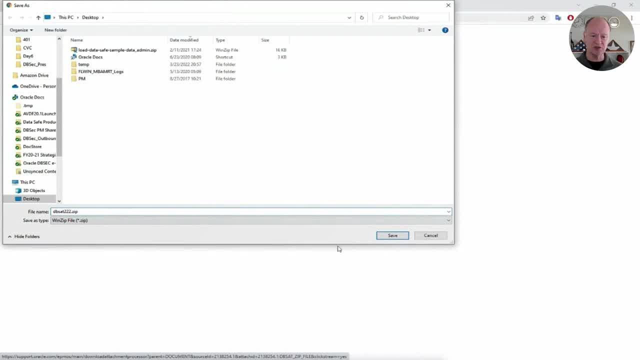 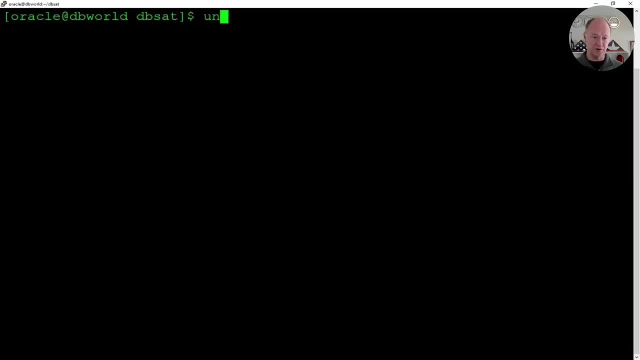 talks about database security assessment tool. We agree that we're going to, you know, abide by the terms and conditions And we download the assessment tool. It's a simple zip file, Very, very easy to use. Once we've got it downloaded, you can see it's a pretty small file. We transfer. 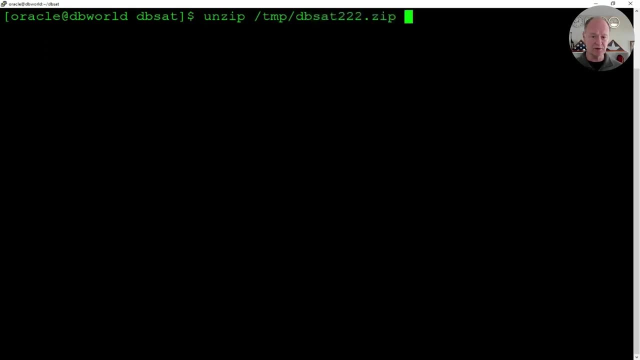 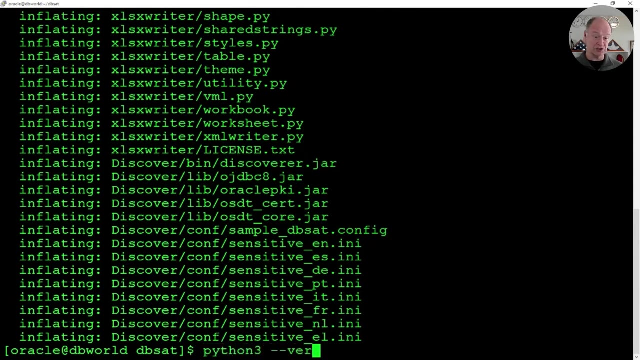 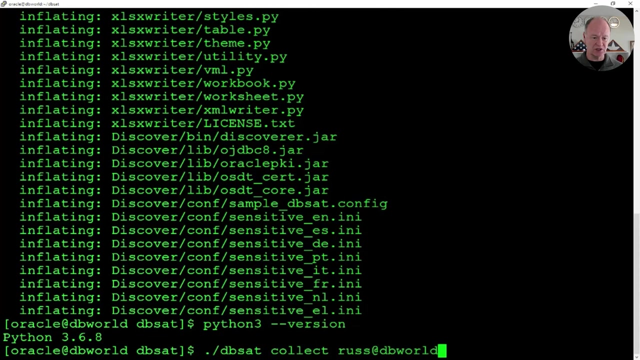 that out to our database server and we unzip it. We've got to make sure that we meet the prerequisites. We need to have Python, We need to have, obviously, the zip and unzip utilities And we need to have Java 1.8.. First we'll go ahead and run the database security assessment. 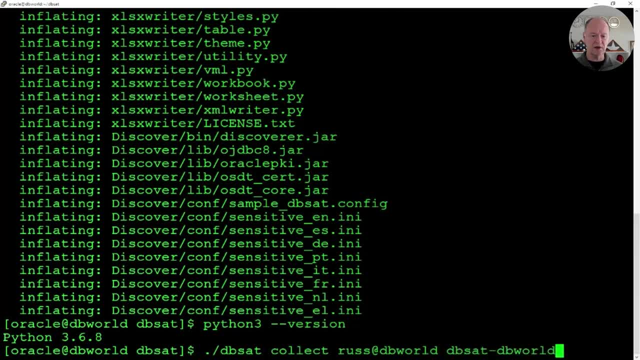 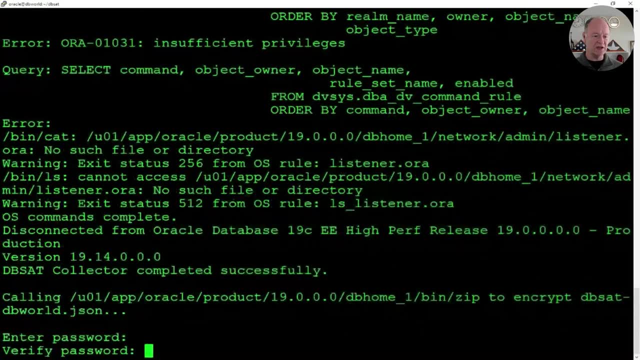 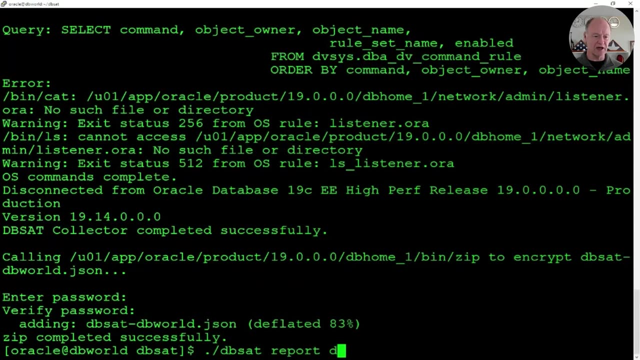 tool collector. We'll give it the credentials to connect to our database and what we want our output file to look at. We give it the password for our database, It runs and then it produces a zip file that we're going to encrypt. That's what the second password is. Next we analyze. 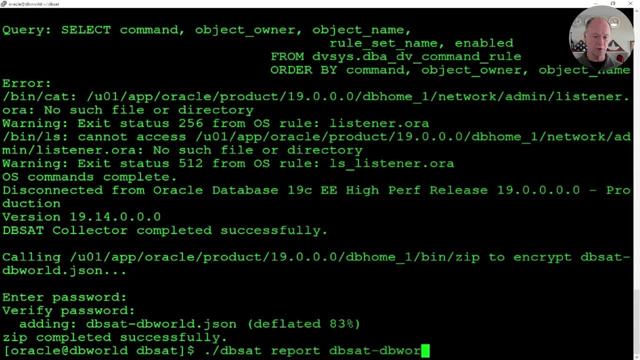 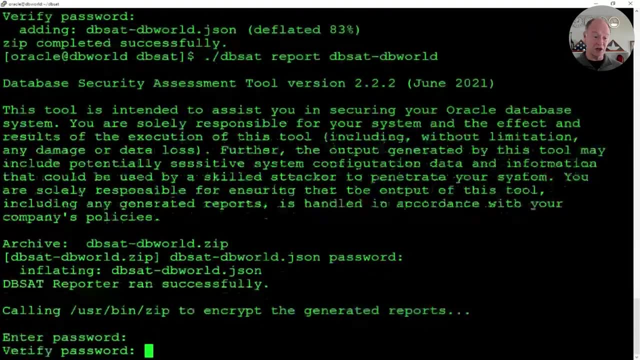 that collected data. We're going to run the database security assessment tool. We're going to run the database security assessment tool. reporter. We tell it where our file is located. We give it the password we used when we created the file. We give it another password This time. 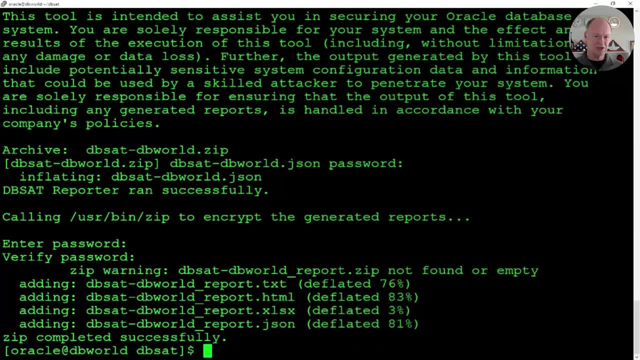 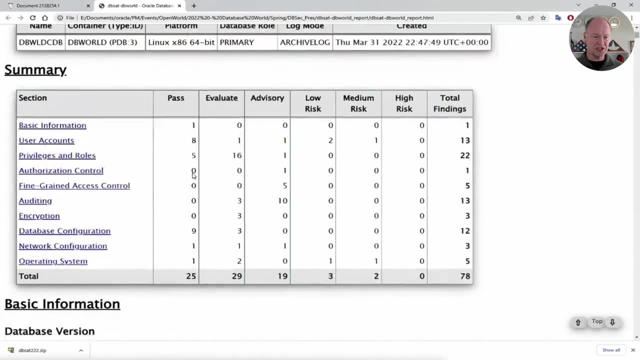 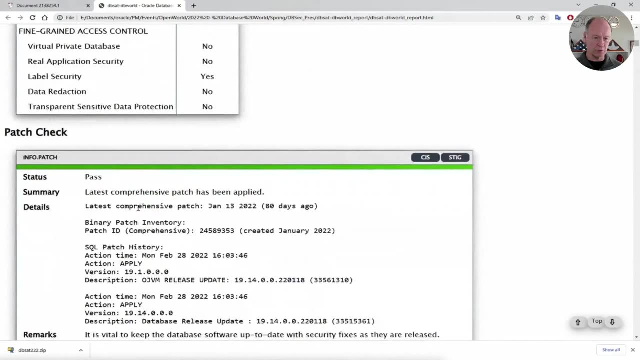 it's going to produce our output file And that includes text, HTML spreadsheet and JSON format demos. We open up the HTML And here you can see an example of what a security assessment looks like. And we've just gone through and we have checked everything from user profiles to the 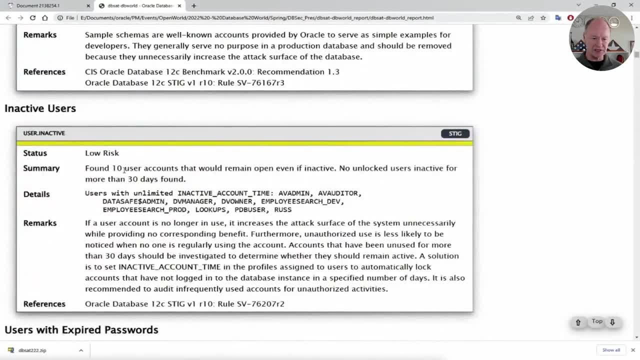 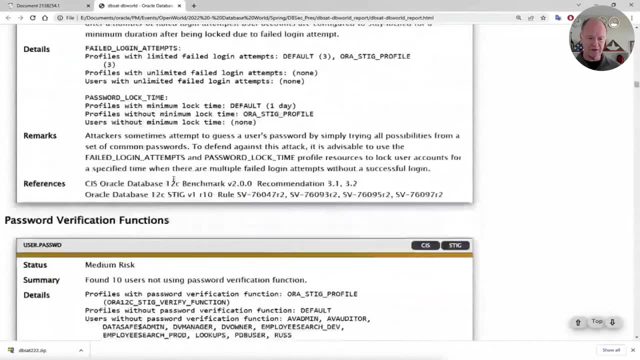 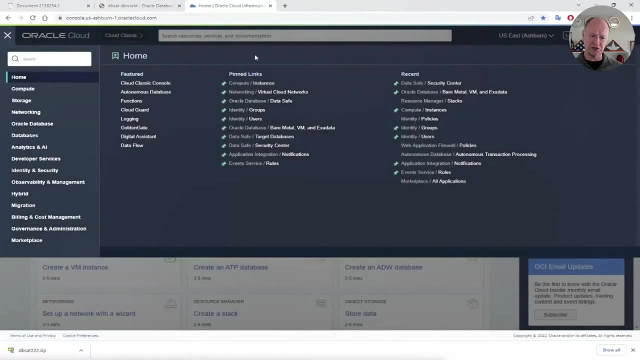 latest patch applied to. how are your passwords being managed, to all those initialization parameters that deal with security, And we tell you we found this area. We think this is an area of risk. In this case, we're looking at something that's medium risk. We have no password verification. 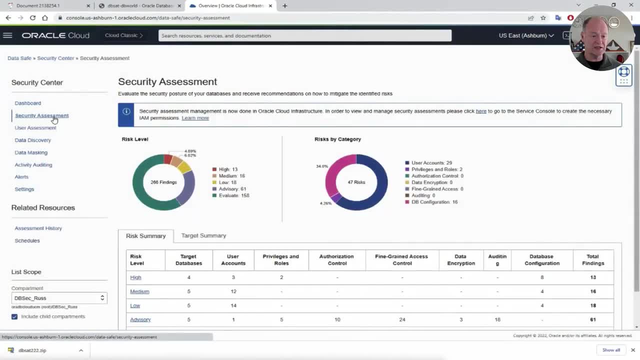 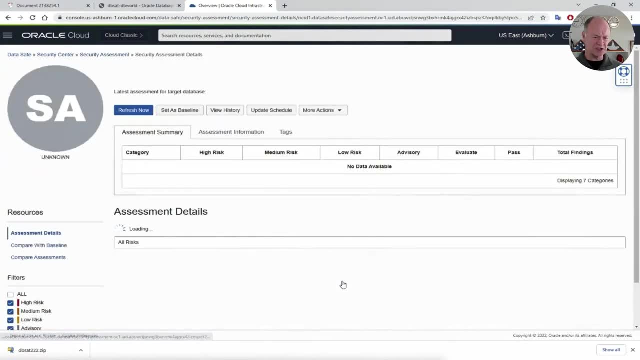 functions. We can also look at this through tools like DataSafe. If you're running in the Oracle cloud, you might be using DataSafe And there you can run a report. You get a little bit nicer dashboard And we can easily compare. 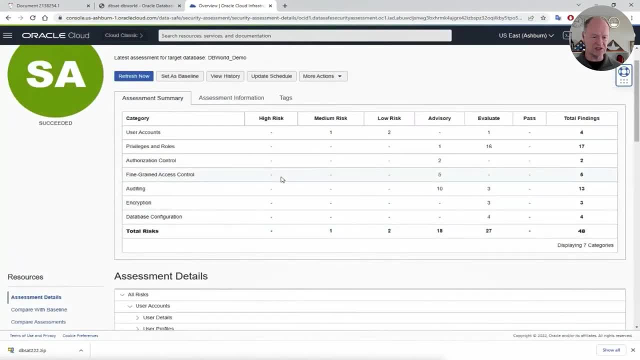 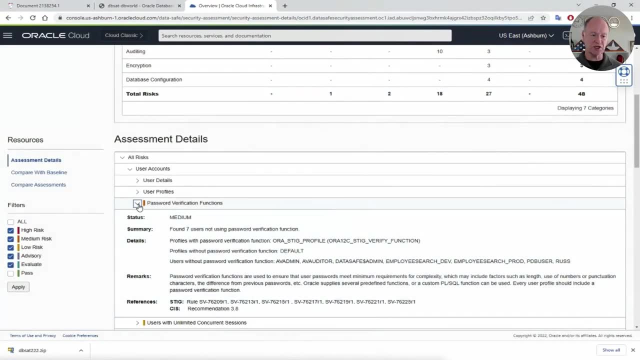 There are assessments from one to another, But these all do the same basic thing: They tell you where you've got risk, where you've made configuration choices that perhaps are introducing risk that you don't need to accept, and give you a clue of how you can back out of. 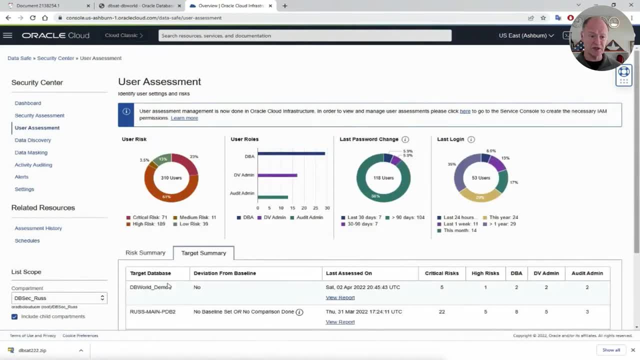 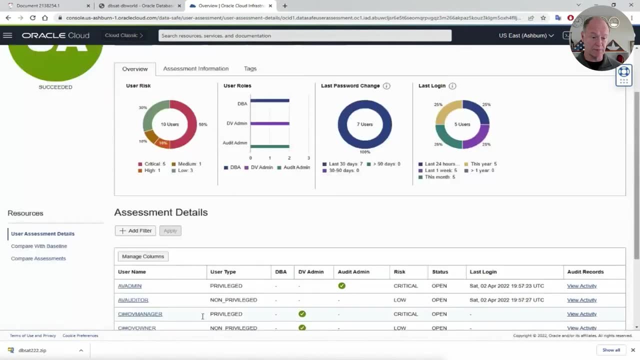 that risk. if you want to, DataSafe has a little bit of extra things in there. For example, we also do user assessment. We look through your users, say which ones are the highest risk if they were compromised, what their access is. You can even drill down and see what their 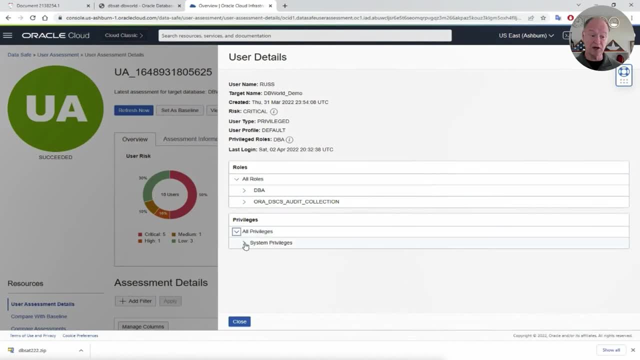 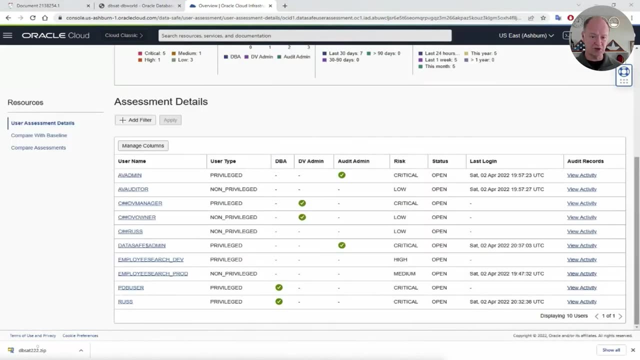 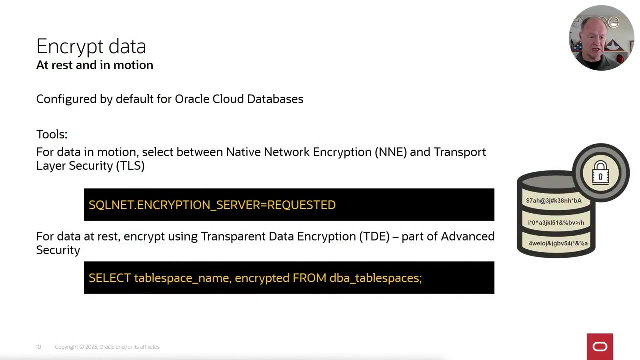 activities are and what their individual privileges are, as well as alerting when new privileges are granted or new users are created. But assessment first thing we do from a security standpoint. Next thing we want to do is encrypt our data. We encrypt our data in motion And for 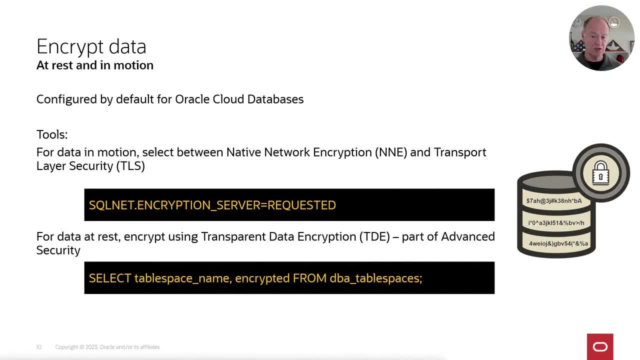 this you have industry standard transport layer security. Transport layer security means that you have to, at a minimum, issue the databases certificate And then you can choose to set up virtual transport layer security where the client also has a certificate, or you can choose not to. 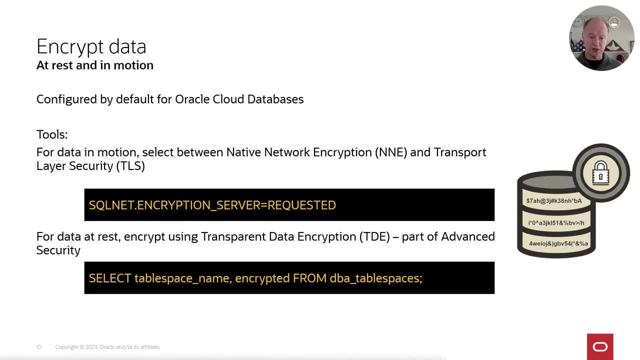 You also have native network encryption, which is old technology, been around a long time, but we do keep it up to date with the latest encryption algorithms- And this allows you to encrypt without certificates. Obviously, TLS with certificates is more secure because the database 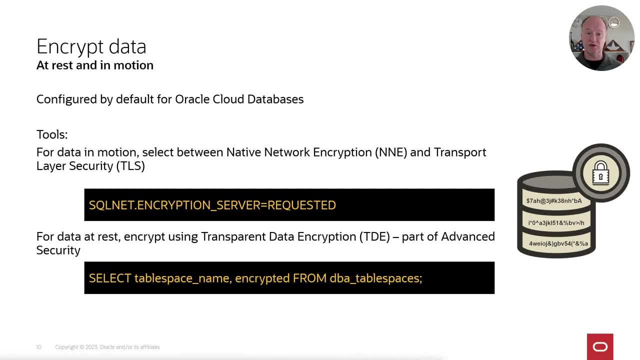 is identified by a certificate, But there are operational things you have to think about when you're managing your data, And that's what DataSafe is all about. DataSafe is all about managing certificates, So, oddly enough, native network encryption is very, very popular. 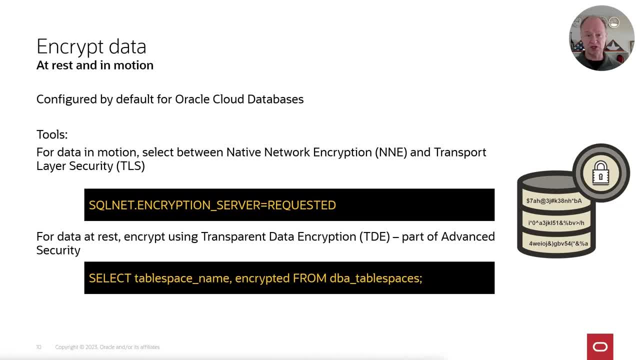 even with security conscious organizations, because you don't have things like the risk of a certificate expiring- All right For data at rest. you're normally going to encrypt using transparent data encryption. Transparent data encryption is one of the features of Oracle Advanced Security, an option for the Oracle database. Let's take a look at encryption and 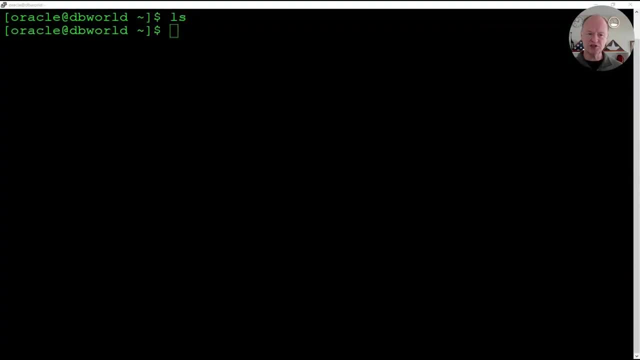 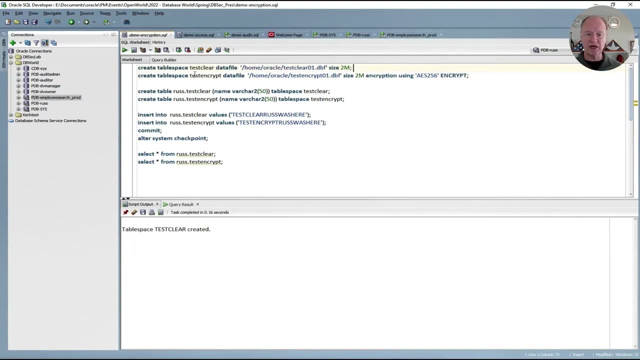 see how this works, And what we're going to do is we're going to start with the database. No user table space is created at all. No real data in there. It's a fresh database. We're going to create two table spaces. One of them is a clear. 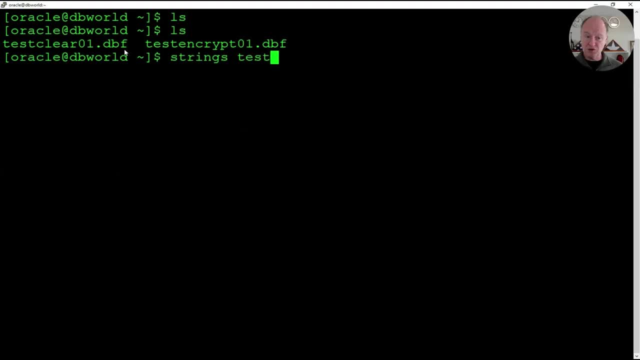 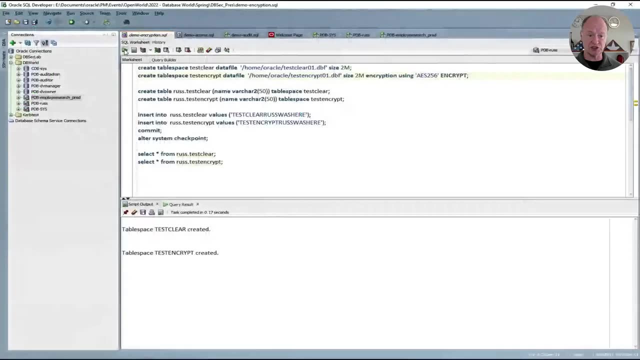 table space One is encrypted. When we look at these two data files for the table spaces, there's no data in the clear table space, no data in the encrypted table space, because we just encrypted it or just created it. rather. Now we're going to create a table in each table space. 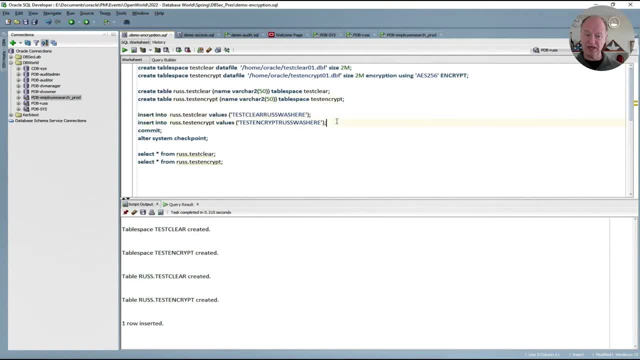 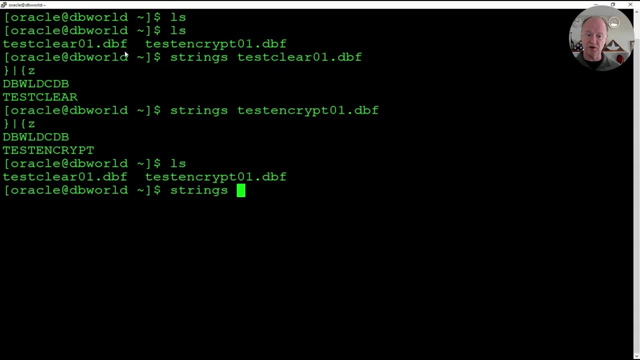 and all we're going to do is create that table and then we're going to insert a single record into each table We're not going to commit, so we still expect to see no data here. We look at the data files, we do a quick strings on it and when we check this, there's no data in. 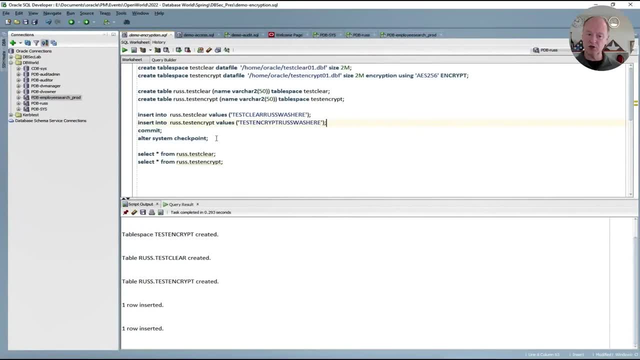 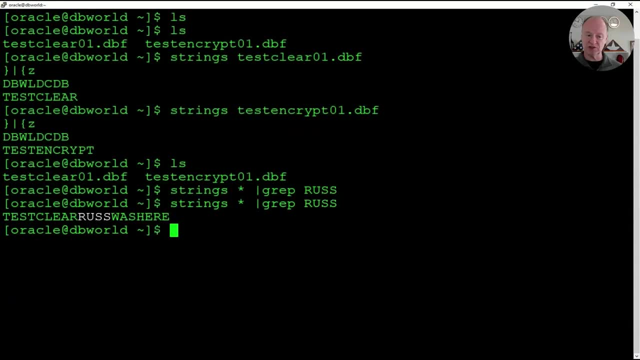 there. This is to be expected. Now we'll commit and do a checkpoint to force the database to write to the files and we'll take a look at our table spaces again. When we look we can see the clear Russ was here. 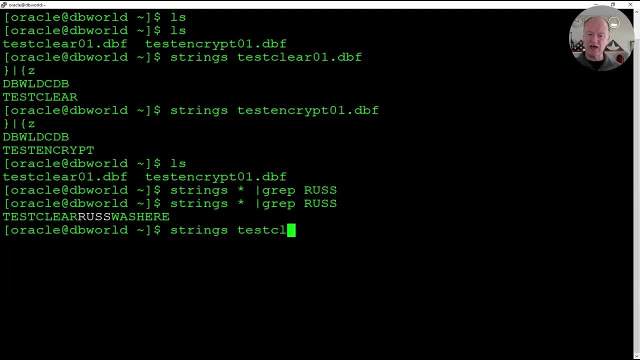 but the encrypt doesn't show up at all. If we look at that clear table spaces data file, there's our test- clear Russ was here. When we look at the encrypted data file- remember there was nothing in there before- Look what we see now: A bunch of gobbledygook. 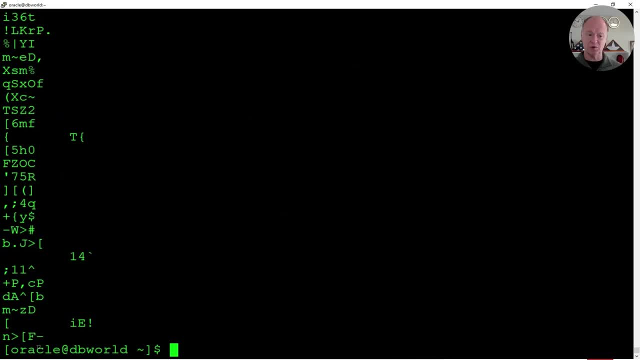 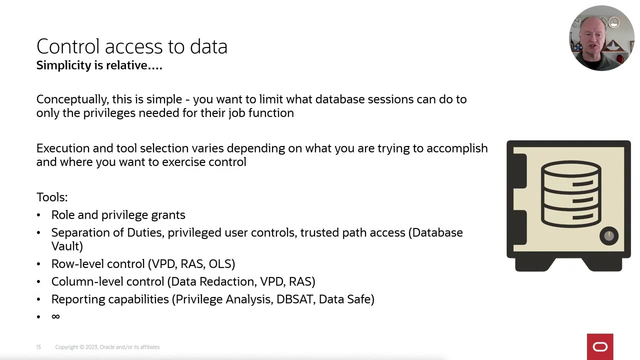 This is encrypted data and this is how simple encrypting the data is with an Oracle database. The third thing we want to do. the third thing is we need to control access to data. This is probably the most interesting thing that you get to work on, because there are so many ways to control. 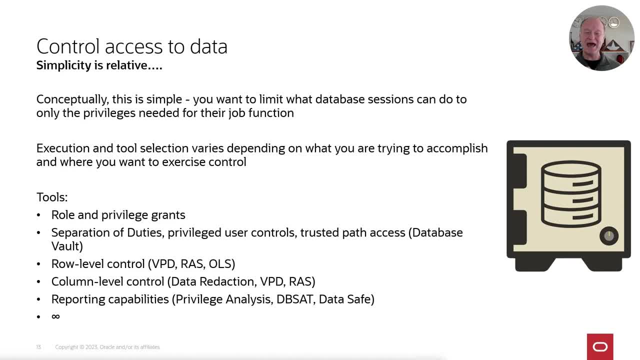 encryption, because there are so many ways to control access in an Oracle database. You can control it based upon data attributes, on session attributes, on objects, on commands. There are so many features to do this, but one of my favorite is something called database fall, and this is 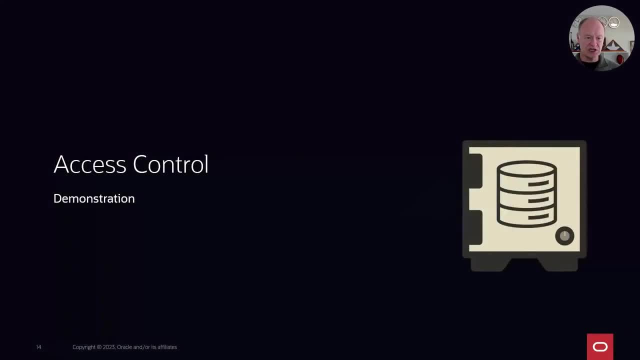 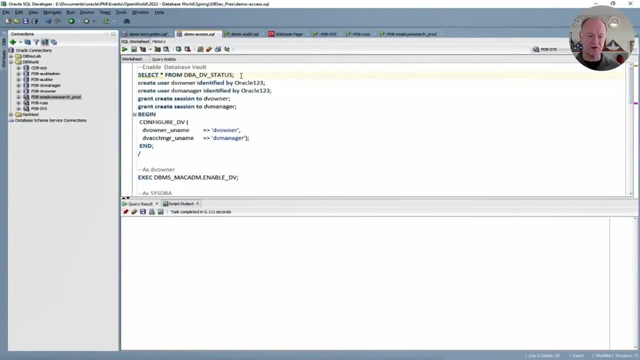 an area where you get a lot of power with the Oracle database. Let's take a quick look at database fall Again. we're going to start with a database where database fault isn't even configured. I'm going to take you from zero to hero in one step Here. we can see no database fault configured. 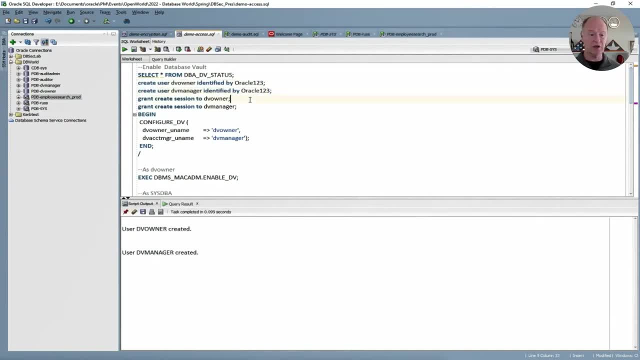 and we will go ahead. We will create a database fault owner and a database fault manager. These are for separation of duties. Once we configure database fault, these users will be used. We'll grant permission for these guys to log in and create a database fault manager. We're going to. 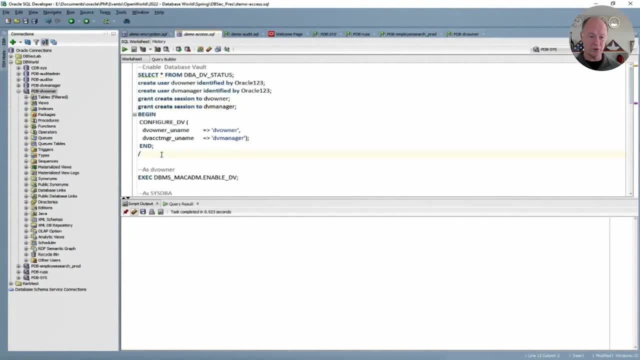 create a session, and that's all we need to do. Now what we're going to do is we're going to configure database fault. Notice that I'm doing this as sysdba. It takes just a second. Then what we're going to do is we are going to log out as sys and log back in as the database fault owner. 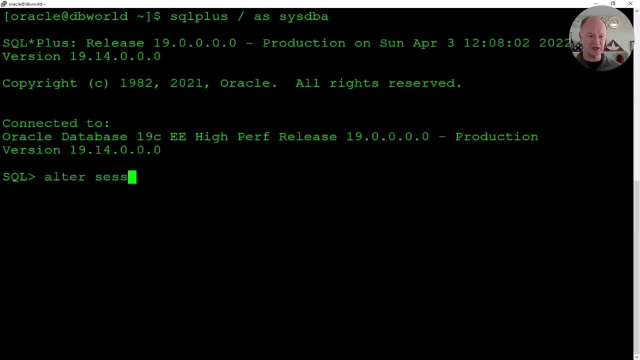 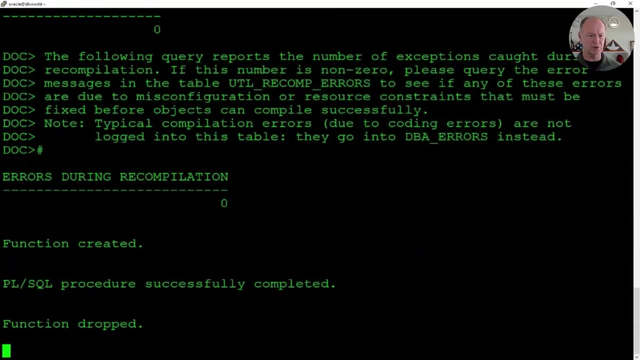 But before we do that, let's go ahead and check to make sure that we've got it, We're in the right container. We'll make sure that we don't have any invalid objects out there, because when we run database fault it does a complete privilege recheck. 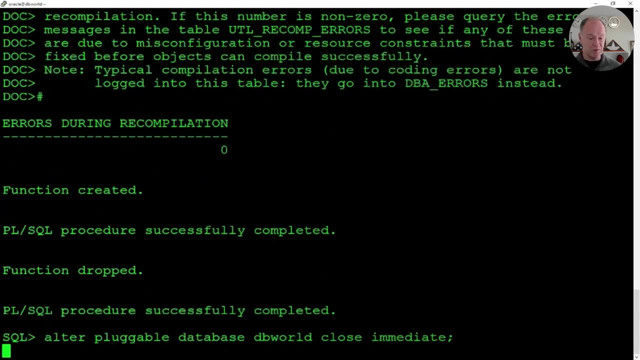 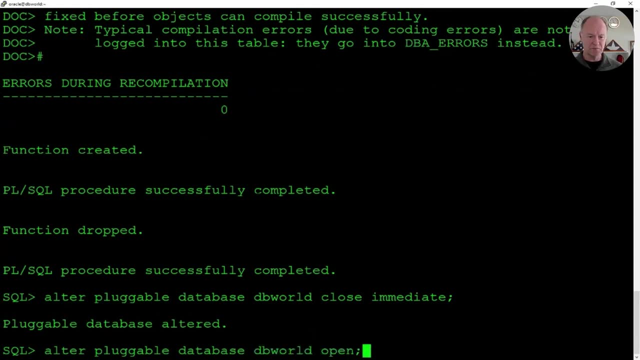 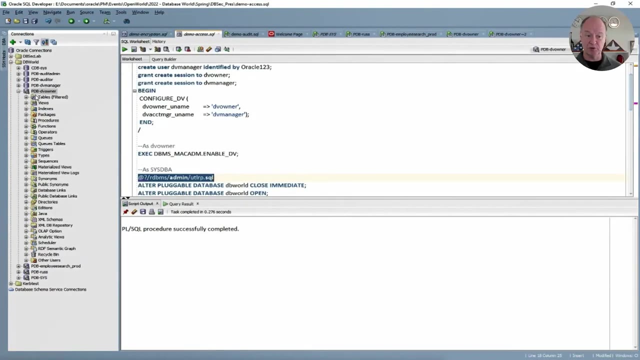 And now we'll close our pluggable database because we've made this configuration change and we want to restart it with the new database fault configuration going. So we bounce our pluggable database. We'll go back to SQL Developer Because we closed and restarted the database. 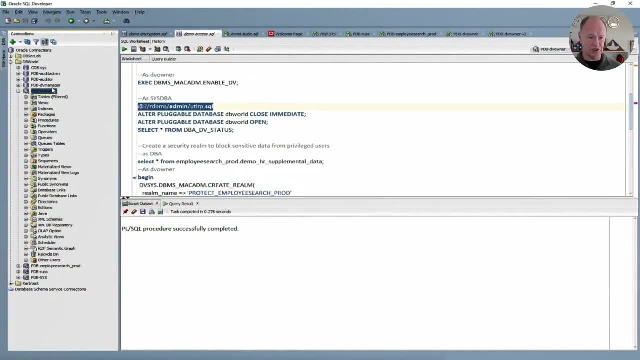 I've got to reconnect, So I'll reconnect as my different users that I've logged in as, And you'll notice that I've got several different sessions here. So make it easy to switch back and forth between sessions here in the demo. Now all we've done so far is enable database fault. That did a few things. It instituted some basic 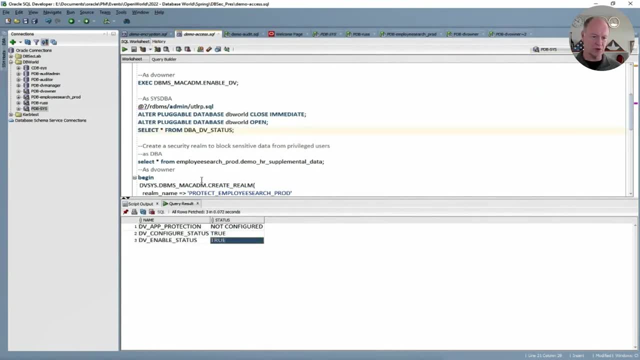 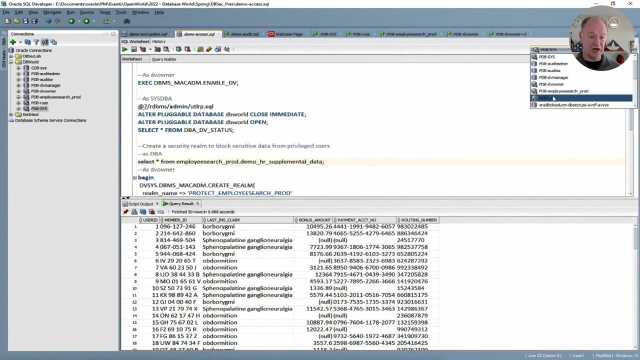 separation of duties. Sys DBAs, for example, can't create users anymore, But I haven't done anything really to protect data yet. So when I go in and I look at a table like this that obviously has some sensitive data in it, I can still see that. I can see that as a DBA I can. 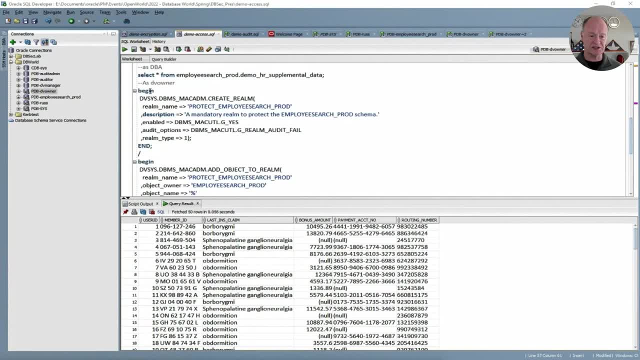 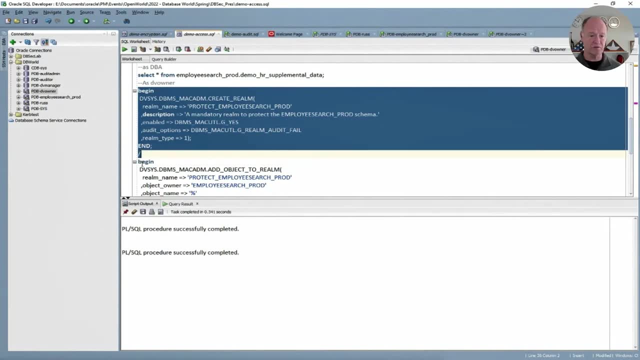 see that as someone who has granted direct object privileges to it And, of course, I can see that as the schema owner. Now I'm going to go in as the database vault administrator and I'm going to put some security around this. The first thing I'm going to do is I'm going to create a realm. 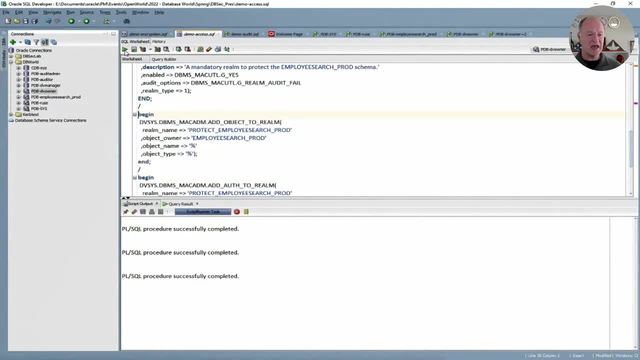 a logical construct to hold security privileges. And then I'm going to go through and I'm going to add the entire application schema to that realm And I'm going to grant only the application owner access to that schema. No one else can see it. And by no one else I mean DBAs, people who have 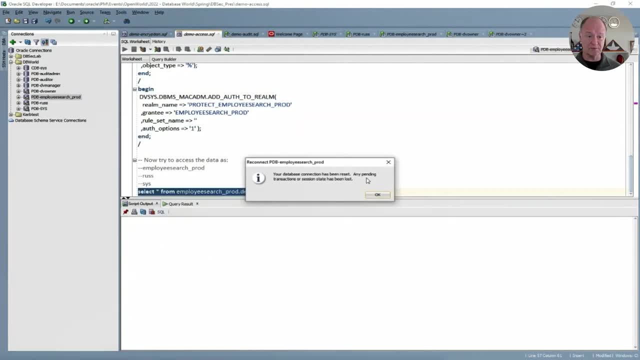 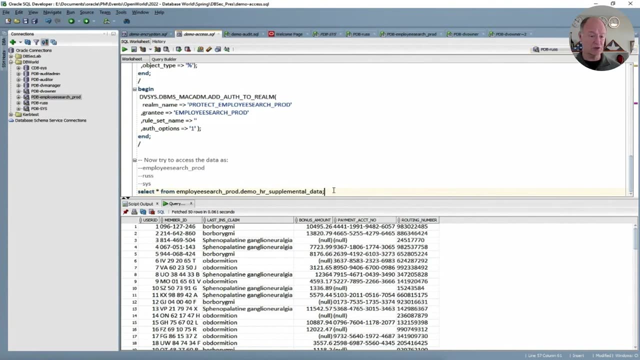 direct object grants Database vault overrides everything. So I'll go in and I will change the schema And I'm going to add the entire application schema to that realm And I'm going to change my session And I'll try logging into someone with direct object privileges. I can't. 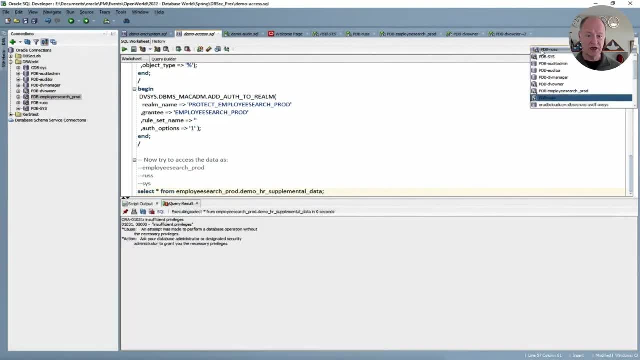 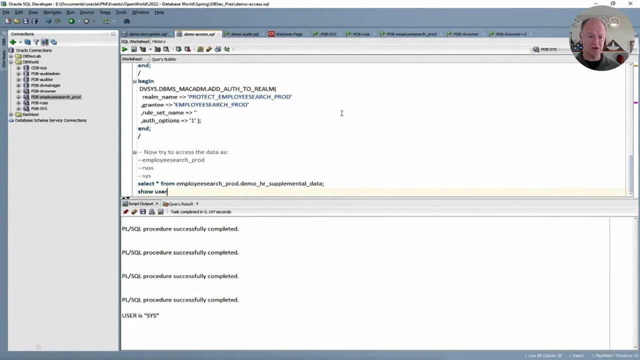 see the data. Okay, Insufficient privileges. I will change and I will become SIS. DBA. can't see the data. And here what I've done is: in just a few minutes, I have protected this application data, which in most cases is sensitive data, from these compromised, privileged user. 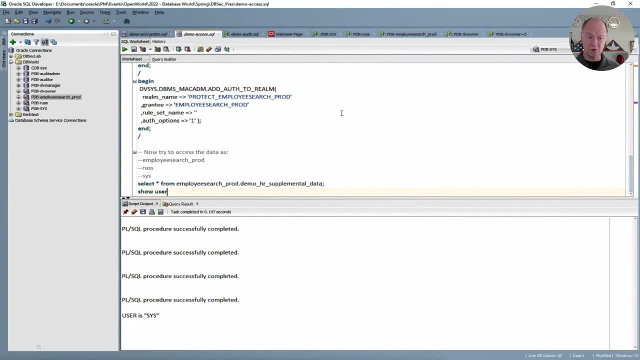 accounts Because you know we didn't really go into a lot of setup for this. but the way most databases get hacked is someone actually compromises an account and just logs in and steals the data, And administrator accounts are the favorite ones to compromise. So here we've. 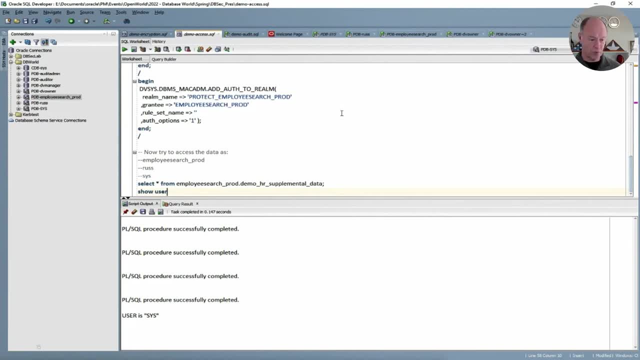 got database vault and we've controlled access. The fourth thing we want to do is we want to make sure that we are auditing what goes on in our database to support those two use cases. One: maybe detect something before it gets out of hand. Two: something does happen. We want to be able to. 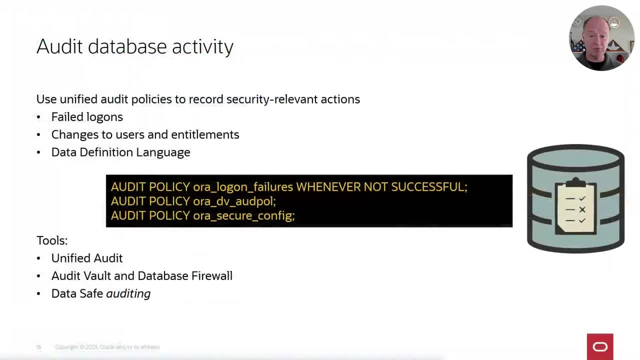 go back and see what happened and what data was accessed. For that, what we're going to use is unified audit. Unified audit was brand new a decade ago back in Oracle 12.. Now it's pretty old, very mature. But what we're going to do is we are going to use unified audit to audit some common security. 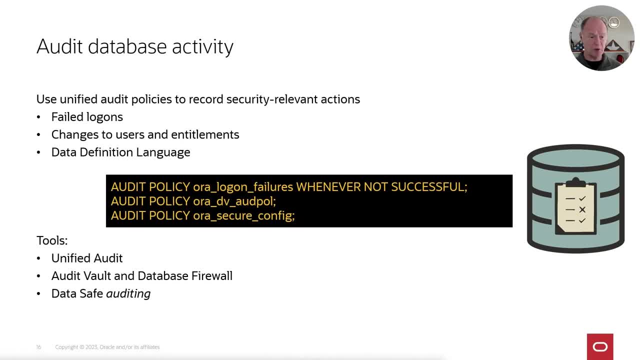 issues. If someone tries to log into the database and fails, well, we want to know that That's a good security event. If someone creates a new user or tries to create a new user or grants roles to that user, we want to know that That's a security event. And if someone is 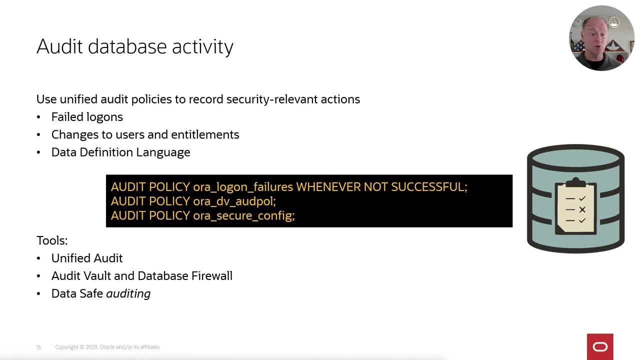 changing structures within the database, changing the definition of the data? we want to know that too. Here our main tool is built in the database- unified audit, But optional tools would include things like Audit Vault and Database Firewall or the auditing capabilities of Data Safe, where 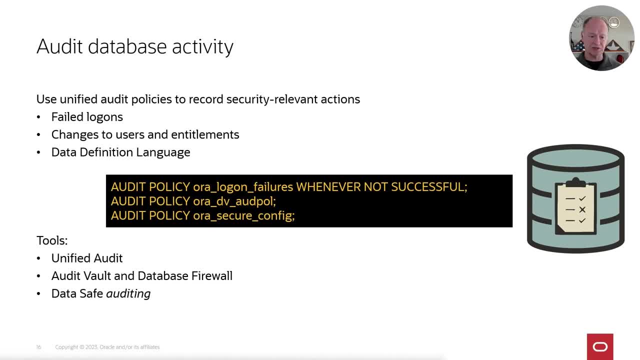 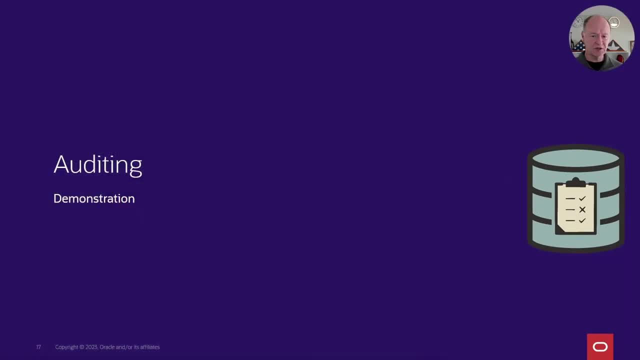 we're going to collect this audit data from the database and move that into a repository for analysis, alerting, reporting, all of that stuff that we need to do from a compliance standpoint. Let's take a look at auditing in action And we'll start again. Clean system. I've purged the 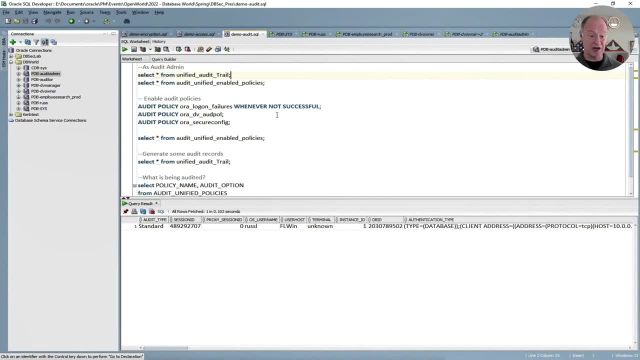 audit trail. There's no real data in there. That one record you see is the fact that I purged it. That always gets audited when you purge your audit trail. But all set to go And what I'm going to do is I'm going to connect to the database as someone with privileges to control auditing. 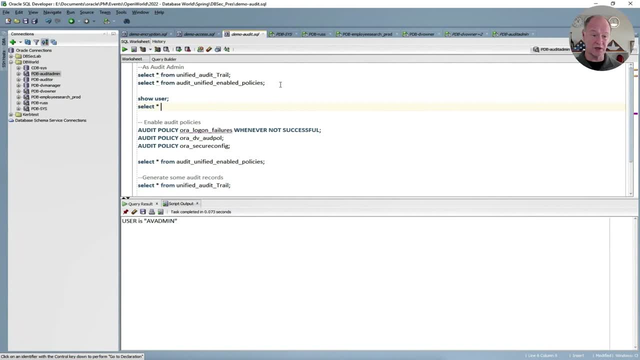 Okay, so you can see I'm an Audit Vault administrator. I'm sorry, I'm an audit administrator. You can see what roles I have And I have that Audit Administrator role And I'm just going to go ahead and turn on three of the default audit policies: logon failures, anything that has to do. 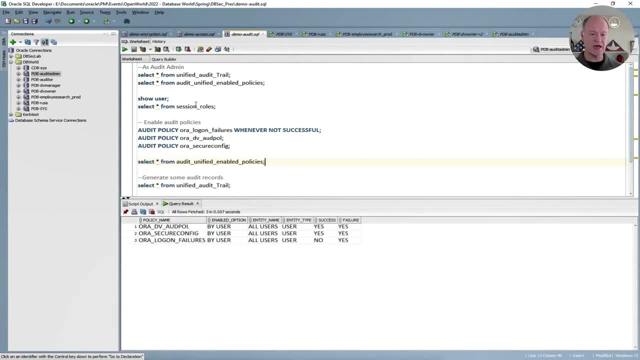 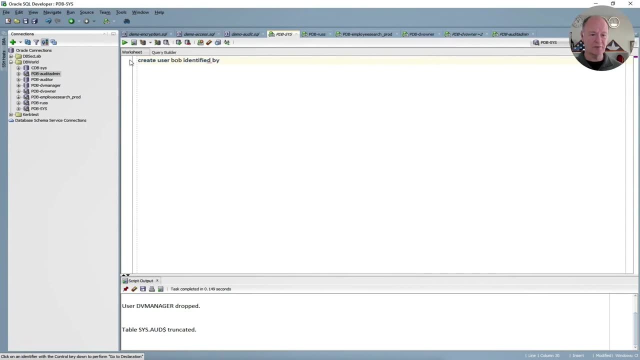 with Database Vault and any of the secure configuration stuff. These are now all active and they're ready to capture activity, So let's create some activity. I'm going to go in and I'm going to try. notice, I'm Sys. I'm going to try and create a user called Bob. Now, remember I turned on. 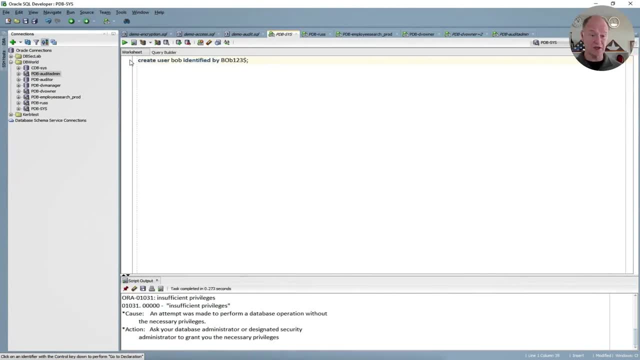 Database Vault, Last piece of security. So this should fail, because DBAs can't create data anymore. And sure enough, it does fail. Generated an audit record. All right, let's see what else can I do. I could try and go in as a different user And this time I'll go in as the Database Vault Account Manager. 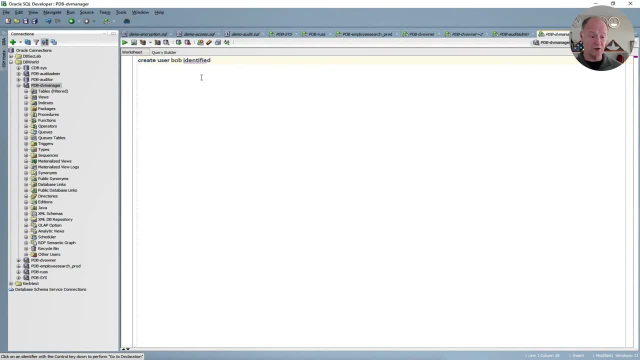 And I will create Bob, But this time because I'm the right user. I do have the privileges under Database Vault to do that. This one, we'll succeed. Again, it's going to generate an audit record, because I set to audit this type of activity. 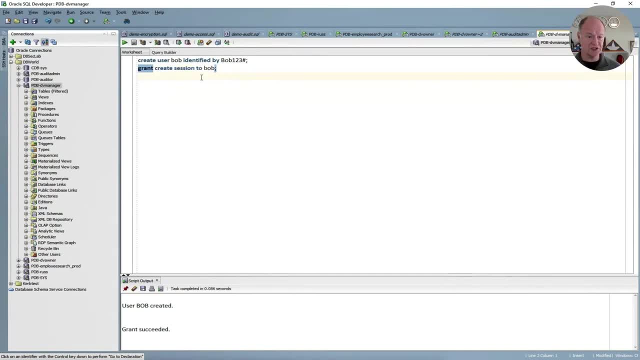 I'll grant privileges to Bob create session. Okay, I'll grant a role to Bob DBA. All of these things are creating an audit trail so that I could see who did it, when they did it, where they did it from, Go back to. 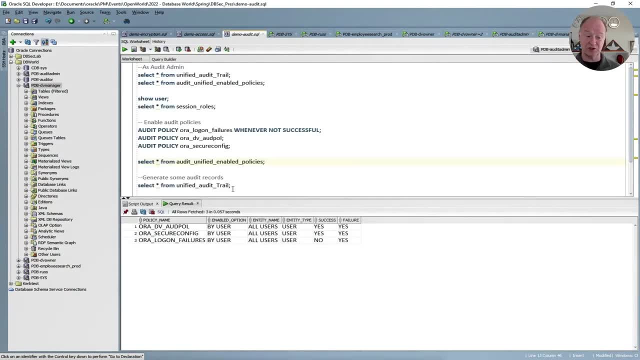 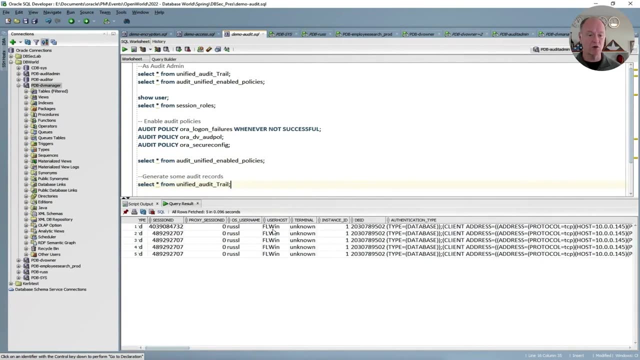 Sys, I'll grant DBA. Before I failed because I didn't have privileges to grant DBA, I was just the user admin. Okay, You can see our DBA, I can see our audit records And when we kind of scroll over and look, it's a pretty wide table. There's a lot of data in. 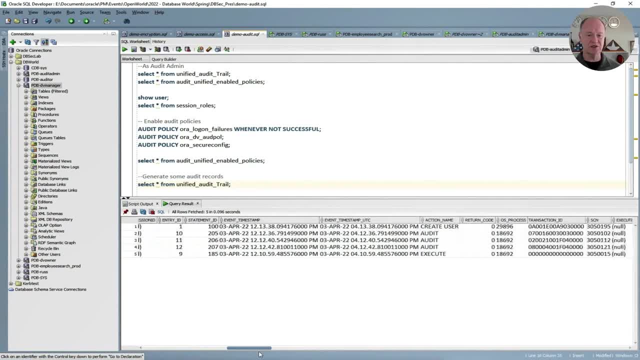 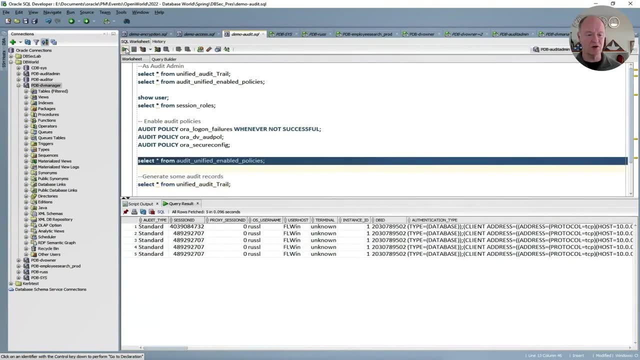 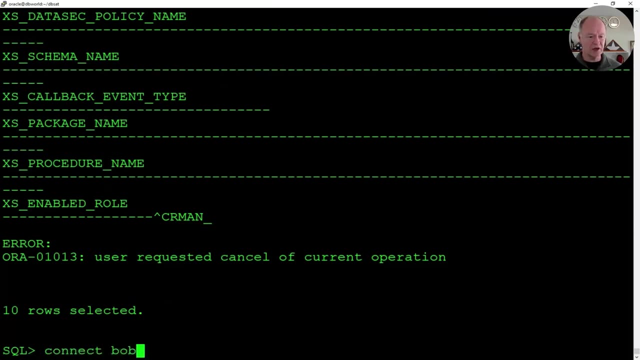 that Audit table. We can see some things were done as the Database Vault Administrator, Some were done as the Audit Administrator, but we can see someone did something to Bob, Someone had a logon failure. All of these things were audited along the way. Okay, Let's do a little bit more. I'm going to try and log into the database. 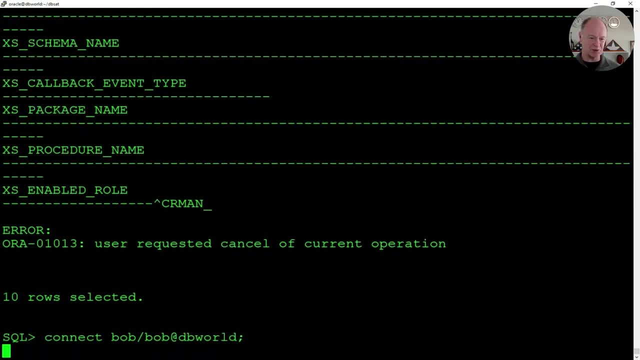 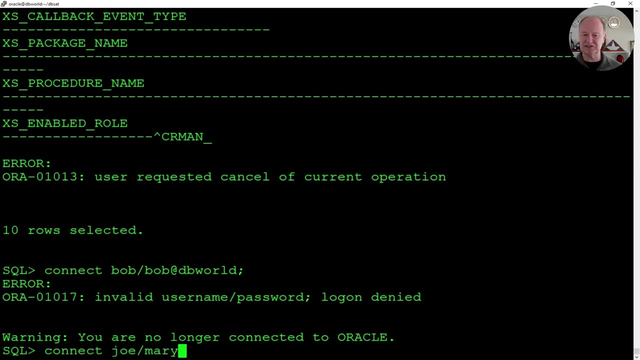 And I'll log in as Bob with the password of Bob, which, of course, is not my password. You watch me use a more secure password when I did this. I'll try connecting as a Joe with a password of Mary, and again, this is not going to succeed because that's not Joe's password and think I've. 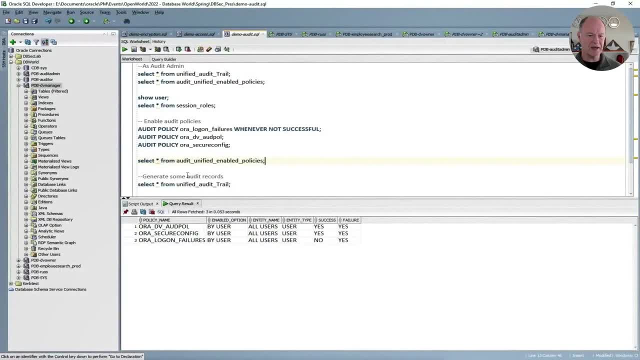 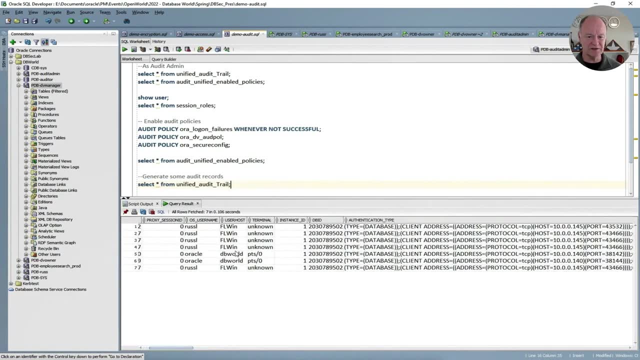 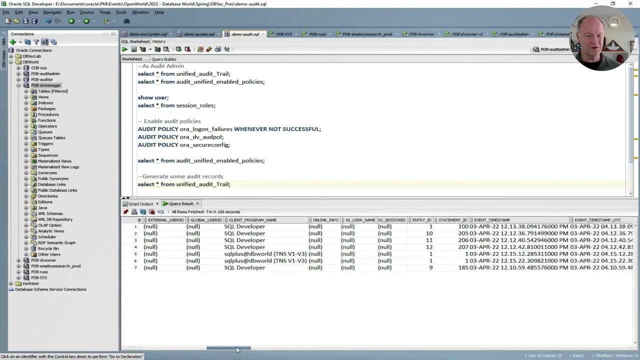 got a Joe in this database, all right. and we go back and again, we look at our audit trail and we can see sure enough, if we scroll over just a little bit, that we came in from a different client as different users and we tried to do different things. if we look in data safe, same type of information is. 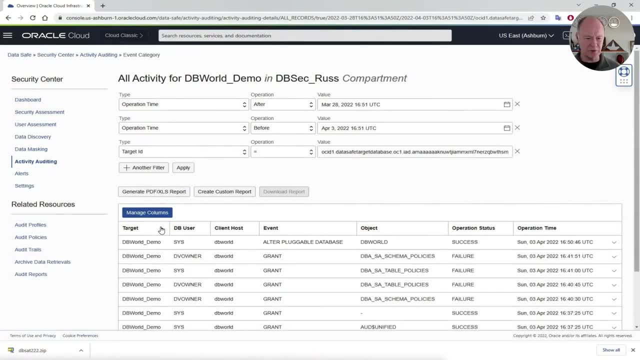 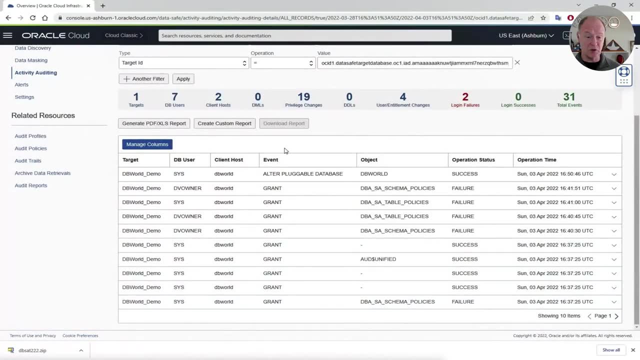 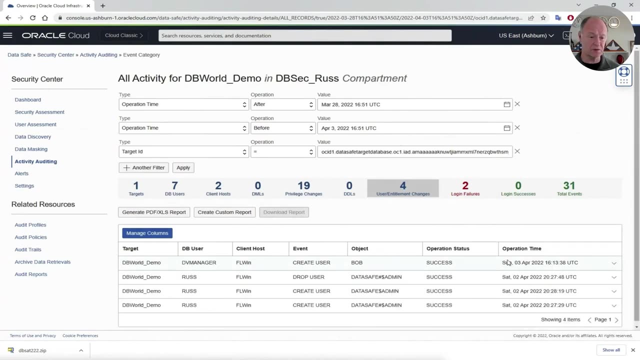 available, but again you get a little bit more with it. you get the ability to generate reports and do analytics a little bit more easily and you can generate alerts when certain things happen. so data safe gives you more to this, but you've got all the tools you need inside of your database, all right. 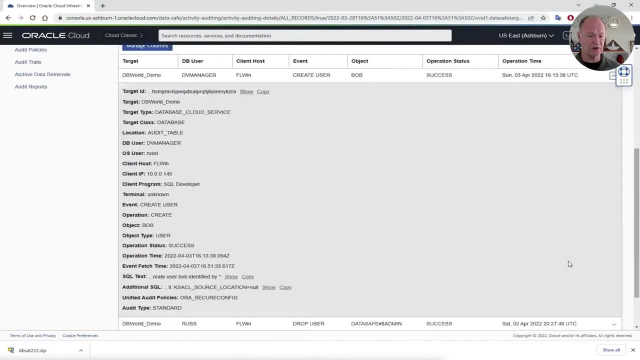 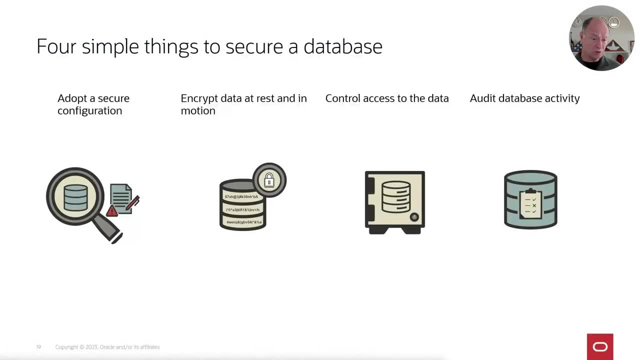 so here's our records- and again you can see that complete record- everything that happened as we were doing our audit activity. all right, so that's it. I told you it was four simple things and it really is four simple things. you need to make sure you understand your configuration, you. 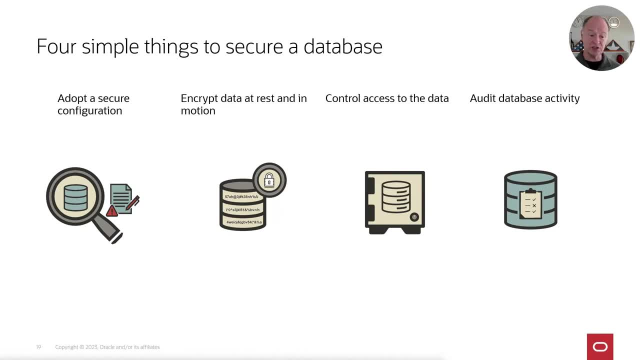 need to monitor your configuration. if your configuration changes, you should be checking it periodically so you know about this. a lot of breaches happen not just because of compromised accounts, but because someone forgot to apply a patch or changed a setting while they were troubleshooting something and forgot to. 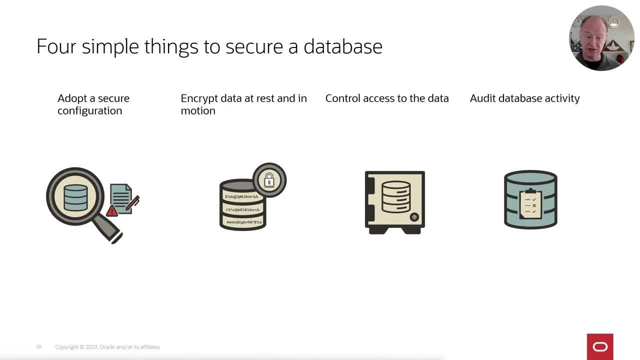 change it back. so check it out if you're not familiar with it. and if you're not familiar with it, I do want to remind you that your, if you're not familiar with it, you can always check your configuration, not as a one-time activity, but as a 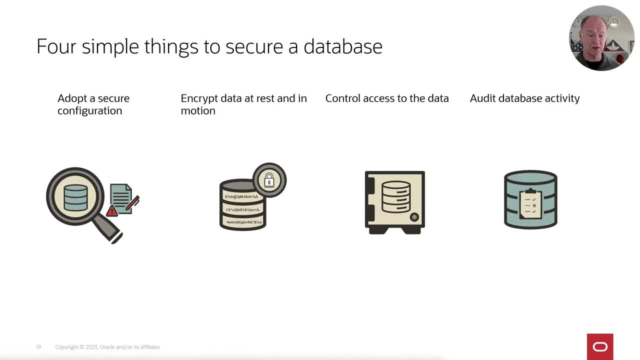 periodic, ongoing standard security process. encrypt your data at rest in motion. data should be encrypted. control access to the data and I showed you one tool: database fault. there are lots of different ways to control access. they have different advantages and disadvantages in use cases. you can spend a lot of time here and finally audit access to your data. I did cheat with one. 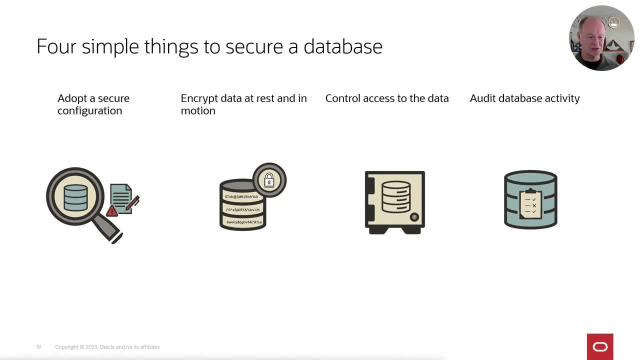 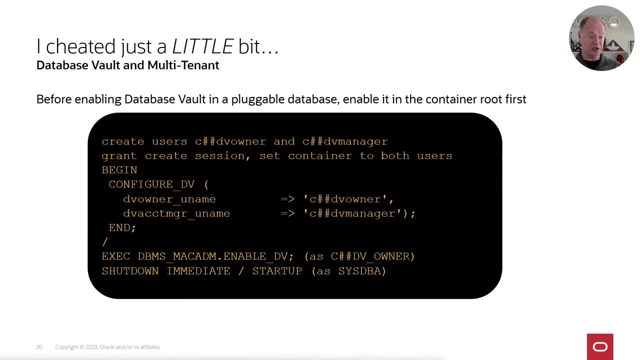 as clean a system as I could. but because I'm in multi-tenant, because I'm using a pluggable database- just full disclosure here- when I enabled database vault, before I had done that, I had already enabled database vault in the container database With multi-tenant. 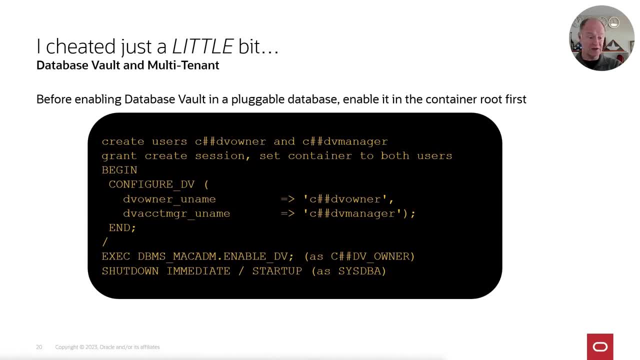 you can have database vault just in the container or you can have it in the container and the pluggable. If you just have it in the container, mainly what you're doing there is preventing container administrators from seeing pluggable data If you have it in the pluggable. that's. 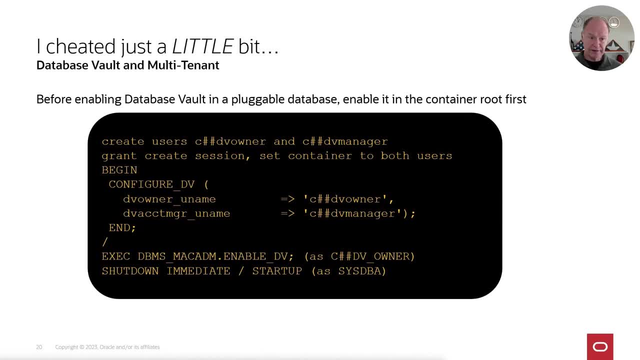 when you get those finer-grained rules, like I was saying, I very carefully when I was talking about auditing- didn't say the fourth and final thing, because there's no such thing as final when it comes to security. There is always more you can do When you've got these four simple 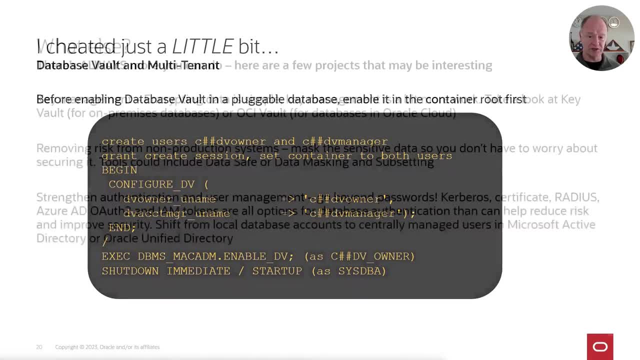 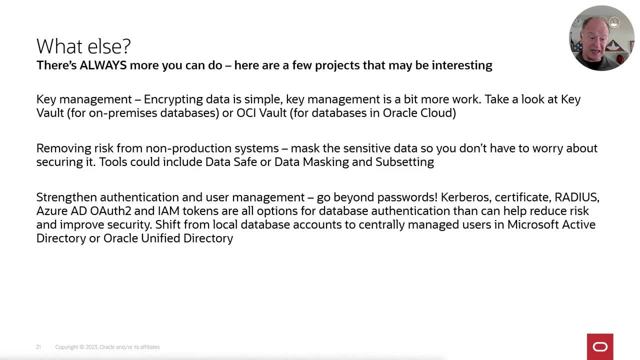 projects done. here are a few other things you might want to consider: Key management for your encrypted data. This is for the data at rest. Encrypting is really easy. It isn't. It is exactly as easy as I showed you. You create the encrypted table space, You put the data in. 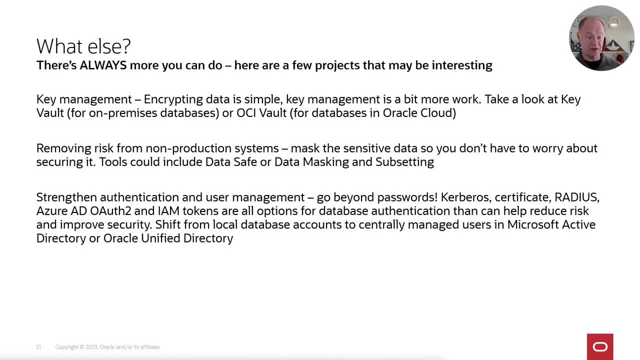 there It's automatically encrypted When you select it. the database automatically decrypts it if you have privileges to see it. Key management takes a little bit more work. The default way that a lot of things store keys is on an encrypted file within the database server. 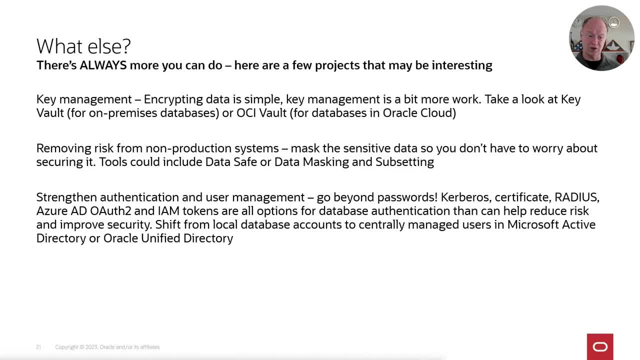 Now think about this: You're encrypting the data to protect someone who has operating system level access from seeing those data files. You're encrypting the data to protect someone who has seeing the data that's in them. Does it really make sense to have the encryption key on the? 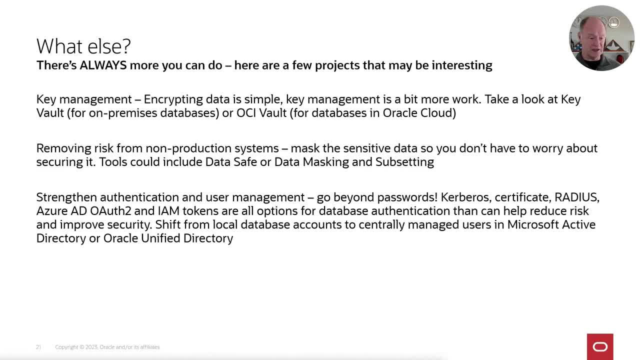 database server? Usually not. That's why you need things like Key Vault so you can move the encryption keys outside of the database server. Take a look at Key Vault if you're on-premises, or OCI Vault if you're running your databases in the Oracle Cloud. A lot of us copy our production. 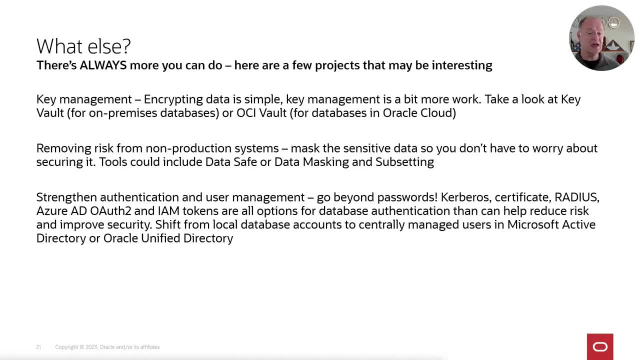 databases back to non-production tested development systems. If you're doing that, you can do everything I just talked about. That may lock down your development system to the point where the developers can't practically use it. Also, evaluators- auditors- tend to be a little bit upset as you begin to proliferate sensitive 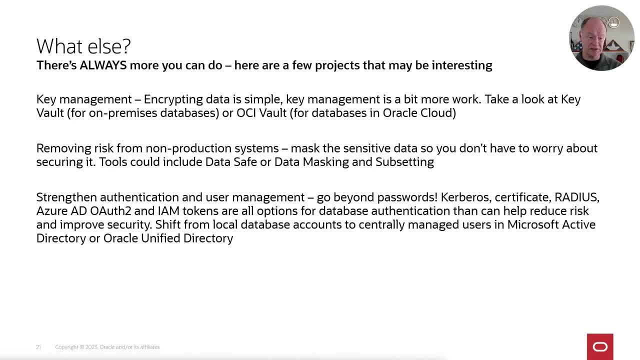 data into multiple repositories, because every time you add a copy of a database, that's just one more chance for that data to be accessed and stolen. A very good security technique is to scramble the data in your non-production copy of the database. Tools that can do this are things like DataSafe. 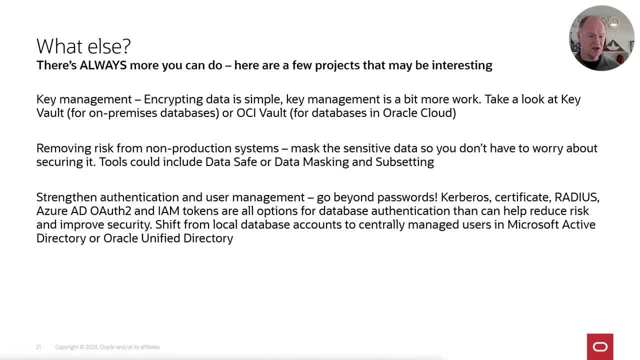 or Enterprise Managers, Data masking and subsetting. And then another project- and this one is really, really popular in today's world- is: take a look at how your users are authenticating. I was showing you username and password, Not the best way to authenticate to a database. Try and go beyond passwords, Your Oracle. 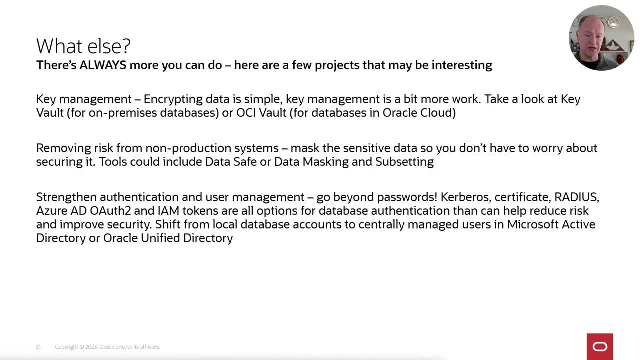 databases support Kerberos authentication, certificate-based authentication Radius, which is a real common way to get to multi-factor authentication. We support tokens. We started doing this a couple of years ago in 19c, Azure AD, OAuth 2 tokens and Oracle Cloud's IAM tokens. All of these are better options for database. 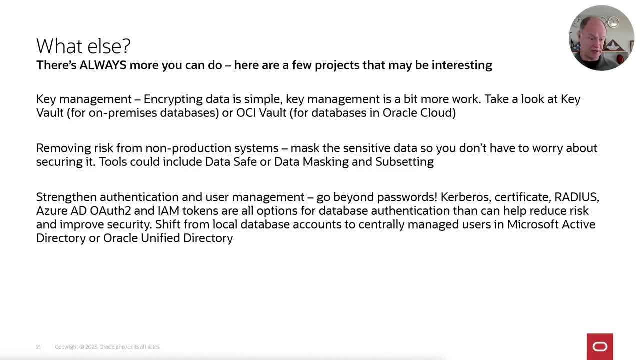 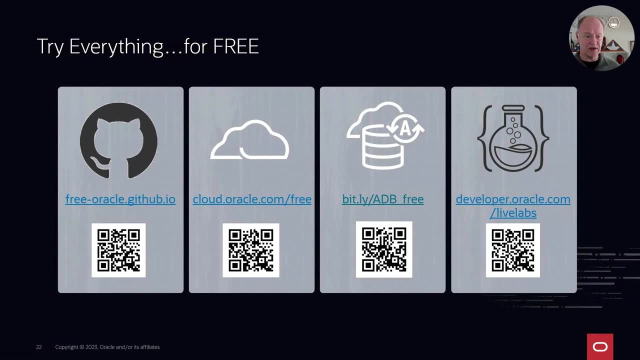 authentication that can reduce the risk that an application account gets compromised or a user account gets compromised and improve your security. So when you can shift from using username and password to stronger authentication. If you want to play around with this, everything I've shown you. 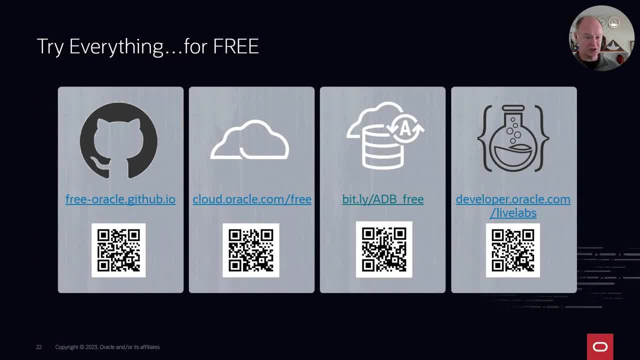 you can get hands-on for free Our GitHub repository. you can find it listed here on the screen. If you look all the way over on the right hand side, you'll see something called LiveLabs. LiveLabs is a wonderful resource, because not just security. 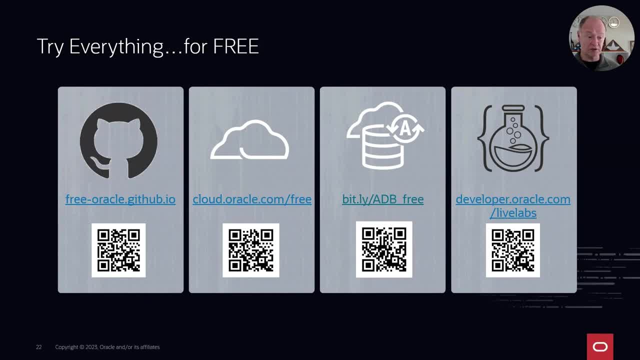 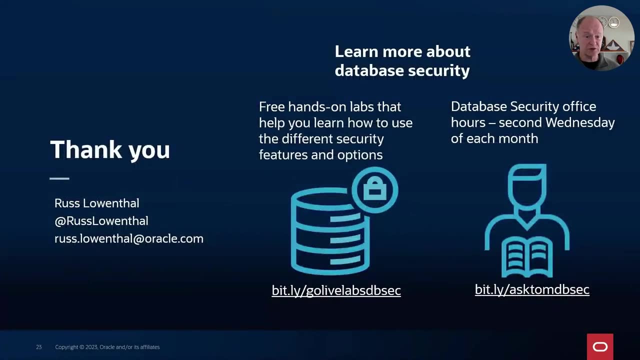 but most things that Oracle can do with the database. there is a hands-on lab out there where you can check an environment out from our cloud on our dime and go through and practice with that environment and learn how to use the features đi. If you're specifically interested in security labs, bitly slash, Go ahead and check out the. 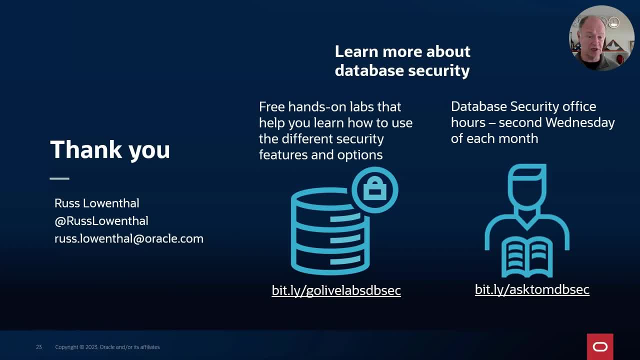 security research. that goes with that. actually, As within the past cycle, Git, Little m-chan trauma is the go live labs. db sec will take you there. and if you really like security, the second wednesday of every month, my team, my product managers, host office hours and bitly slash. ask tom: db sec is. 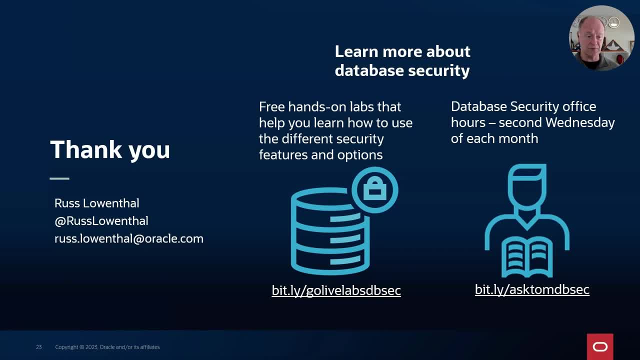 how you can find out what the schedule is for the office hours, what the topic is for that month. if you can't attend live, you know it's a global, global world and you could be sitting somewhere around the world from where we're doing this and the time we're holding office hours isn't. 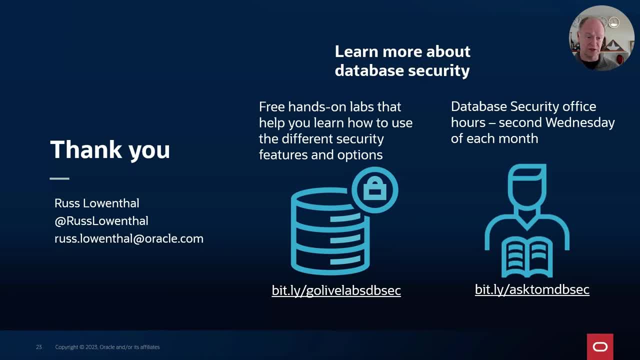 convenient to you. don't worry, we record them. we post the recordings a couple of days after the event and you can always go back and see what's going on with it. thanks for joining us. if you'd like to again, if you, if you like security. these are great resources for you. all right, and that's. it. thank you again for giving me your time today.